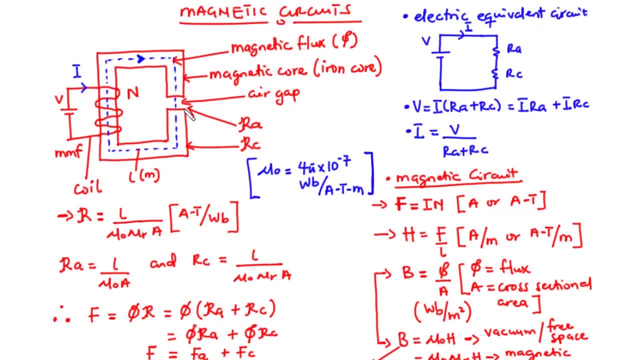 the ion core as well as the air gap. Now let's focus on the electric equivalence of this circuit. So here we have a voltage source V that is driving current Ci through the circuit, and the resistance of this circuit is made up of the resistance as a result of the air gap, as well as the resistance. 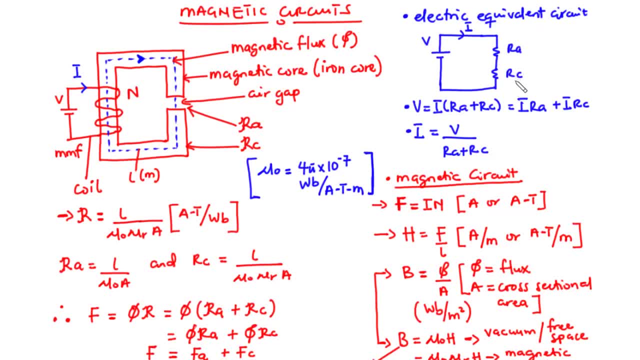 as a result of the ion core. So we know that the applied voltage or the source voltage is giving us the current that flows through the circuit times the total resistance. that is according to Ohm's law, And that is equal to multiplying I across. then you have: I times Ra plus I times Rc, and thus 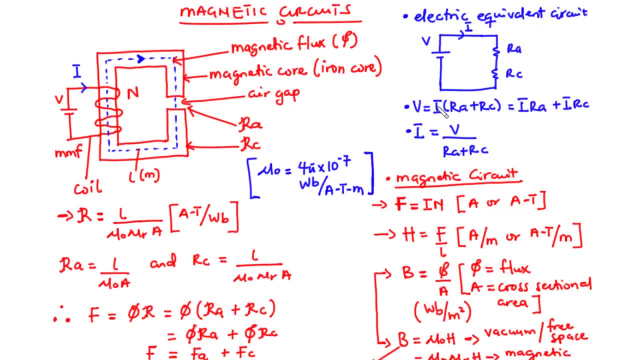 the voltages dropped across the circuit is equal to the source or the applied voltage according to KVL, And if you want to find the current flowing through the circuit, then that is equal to the applied voltage divided by the total resistance. Now coming back to the magnetic circuit, 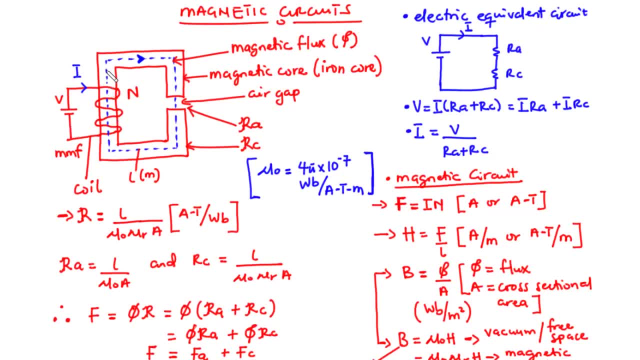 the force or the source that drives magnetic flux within the circuit is called the magnetomultiforce, which is represented as MMF, And then within the magnetic circuit we have two resistances, that is, the resistance as a result of the air gap, as well as the resistance as a result of the ion. 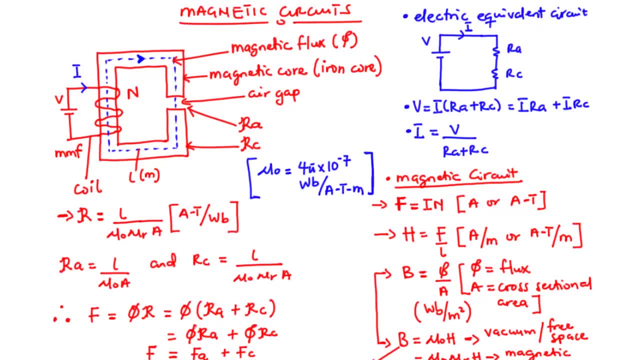 core, Now in a magnetic circuit. we call this resistance the resistance of the magnetic flux. In the magnetic circuit. how far inside is the air gas? or the resistance of the ion core? Directly, the resistance of the ion core is represented as ToV, kinetic Kerr, prime of mate And of. 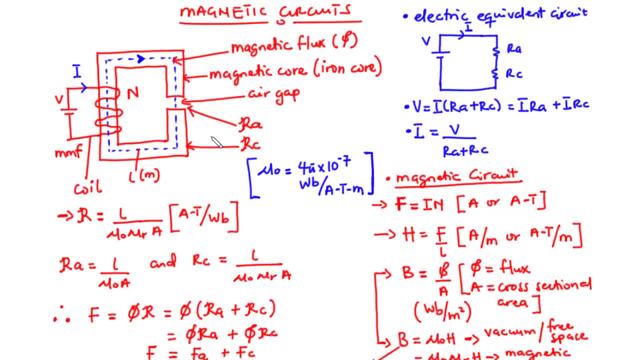 has a high reluctance and a low magnetic permeability. Now, given a magnetic circuit, in this case, the magnetomotive force, or better still, the MMF that drives magnetic flux within the circuit is given by F, which is equal to the current in the core times, the number of turns of the core, and that is measured in amperes or better. 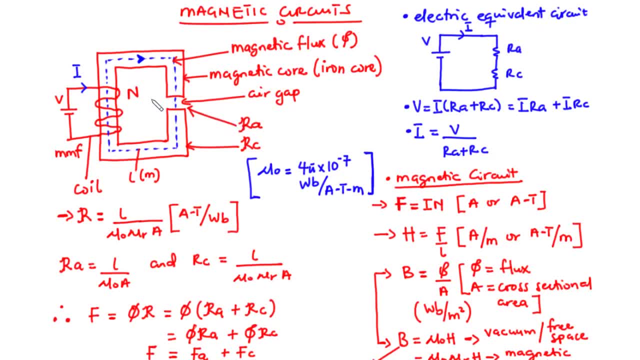 still ampere- turns. Now, as the flux flows through the magnetic circuit, a magnetic potential drop is developed across each section of the circuit, and if the circuit is homogeneous and thus has uniform cross section, then what this primarily means is that the magnetomotive force, or better, 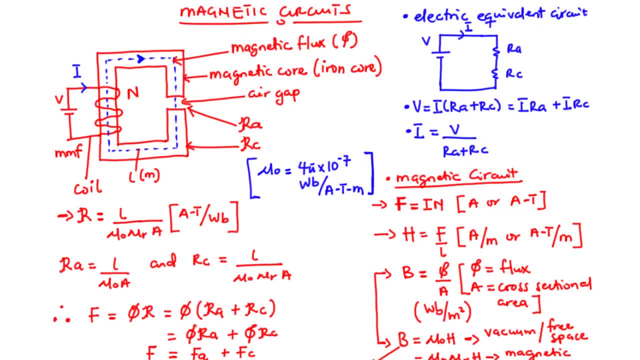 still the MMF per meter length of this magnetic circuit is said to be the magnetic field intensity and that is represented as H and that is equal to the MMF divided by the length of the magnetic circuit and that is measured in amperes per meter or ampere turns per meter. 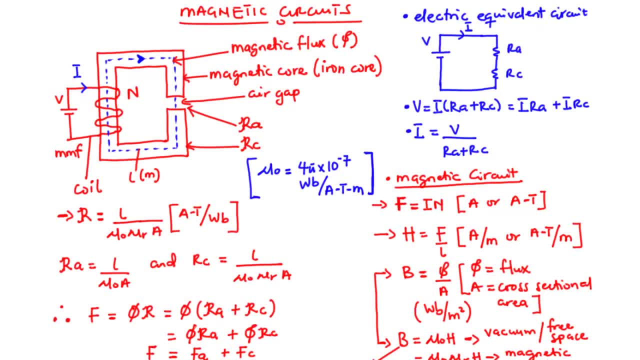 Now we also have what we call the magnetic flux density, which is equal to the magnetic flux divided by the cross sectional area, also measured in Wb per meter square. and then this magnetic flux density is measured in Wb per meter square. and then this magnetic flux density. 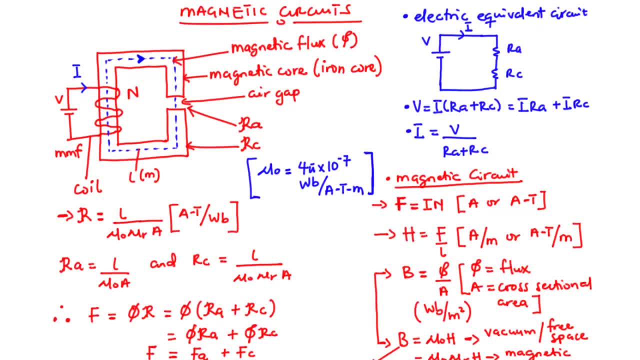 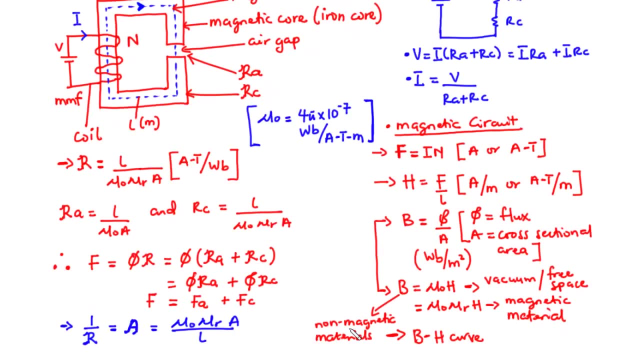 is somehow related to the magnetic field intensity. by this formula, that is, B equals mu naught times H, and then we can use this formula to find either B or H, especially when we are dealing with non-magnetic materials or, better still, free space or vacuum. 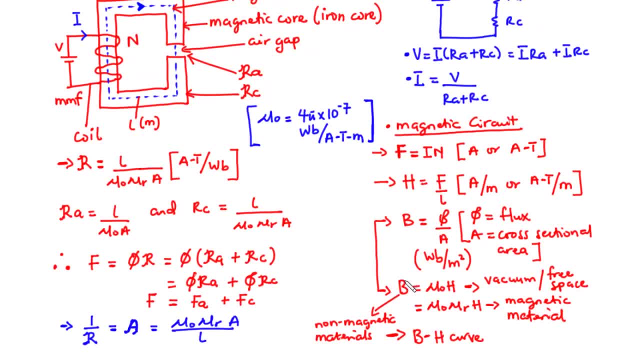 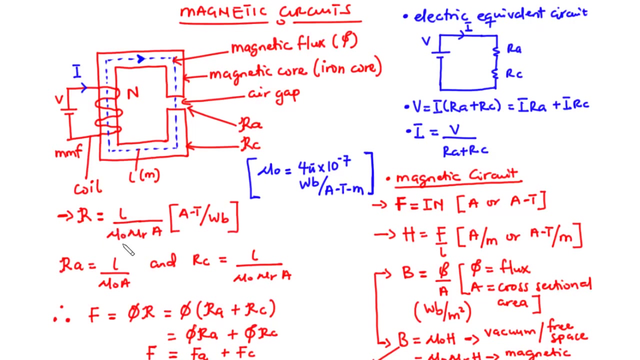 Now, in the case where you want to find the value of either B or H for a magnetic material, you can't use this formula. hence it is advisable to use the BH curve to find either B or H when one of them is known. Now the reluctance of this circuit is given as L divided by mu, naught, mu, R A, where L is. 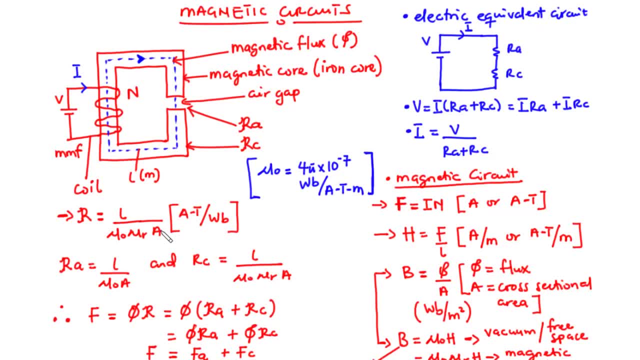 the length of the magnetic circuit, and then A is the cross sectional area, and then the reluctance of the magnetic circuit is measured in amperes per meter square. Now we can use this formula to find either B or H, when one of them is known. 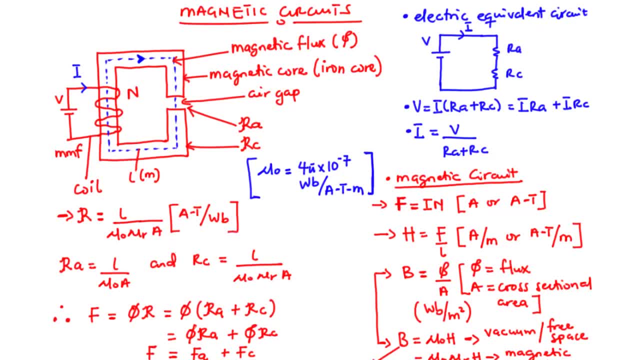 Now the reluctance of this circuit is given as L divided by mu naught, mu R A, where L is the distance in distance per Weber. and then, considering this circuit, now the reluctance as a result of the air gap is given as L over mu naught A, where the reluctance as a 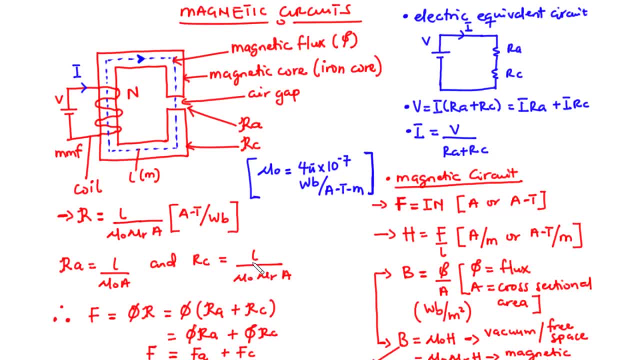 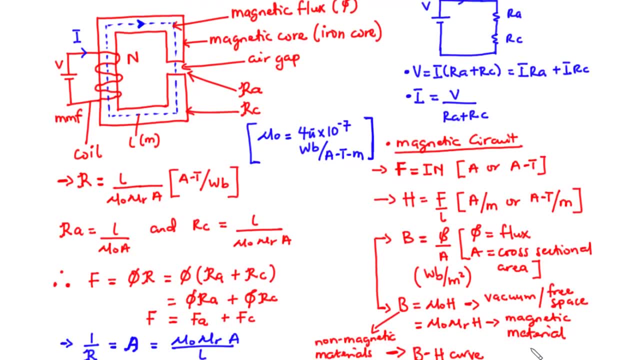 result of the ion core is given as L over mu naught mu R times A. Now from Ohm's Law we know that the source voltage is equal to the current times the total resistance. that is considering an electrical circuit. Now, in the case of a magnetic, 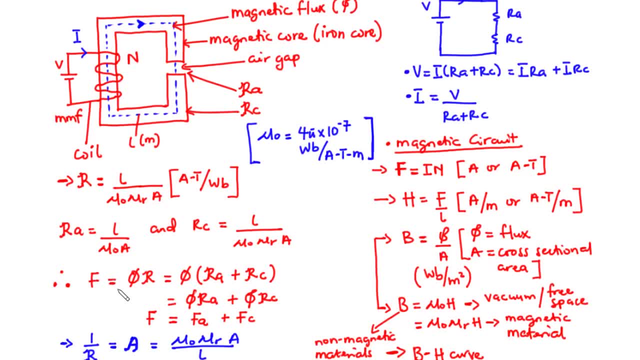 circuit, the magnetomotive force F is equal to the magnetic flux times, the total reluctance. In this circuit we have the total reluctance composed of the reluctance as a result of the air gap and the reluctance as a result of the magnetic core or, better still, the ion core. Now, if you should multiply the flux, 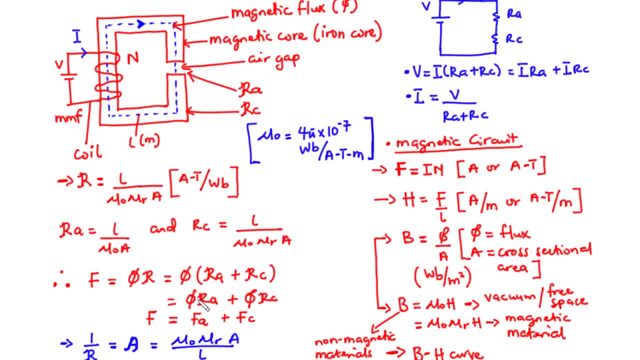 by Ra and then Rc, then you are going to get flux times Ra plus flux times Rc, and that becomes the magnetic potential drop as a result of the air gap plus the magnetic potential drop as a result of the ion core. Now, if you should add these, 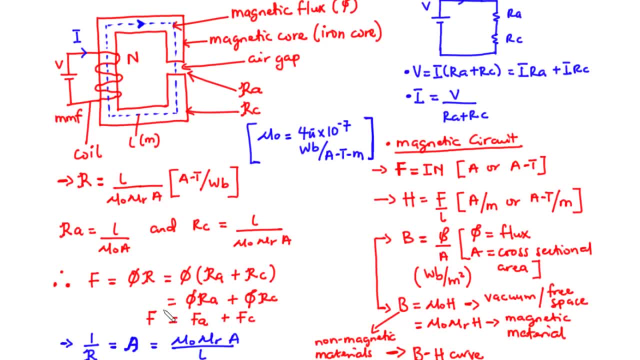 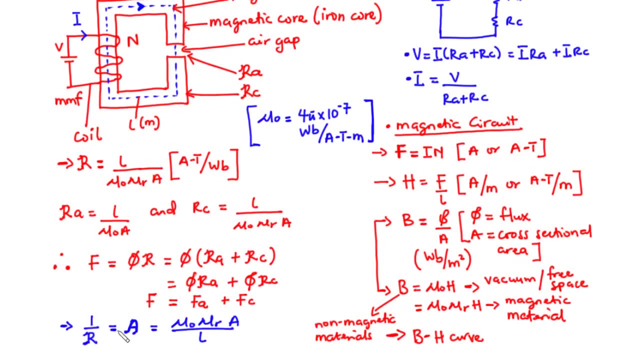 two values, then that should be equal to the magnetomotive force. Now, what do you think will be the, the inverse of the reluctance? Now, the inverse of the reluctance is called the permeance, and that is equal to mu naught mu R times A, divided by L and this: 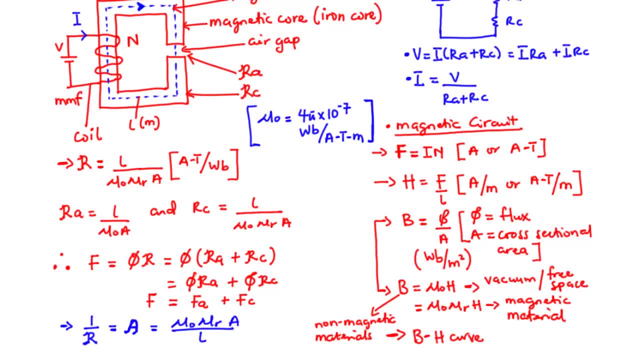 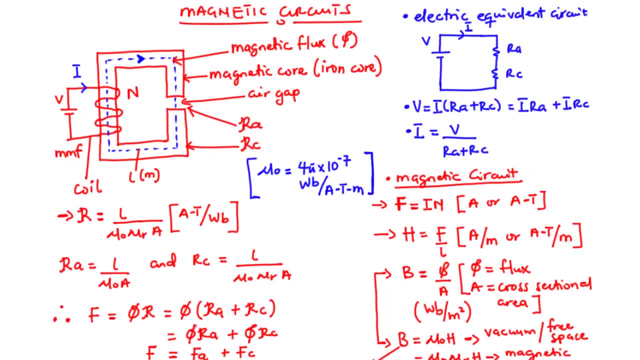 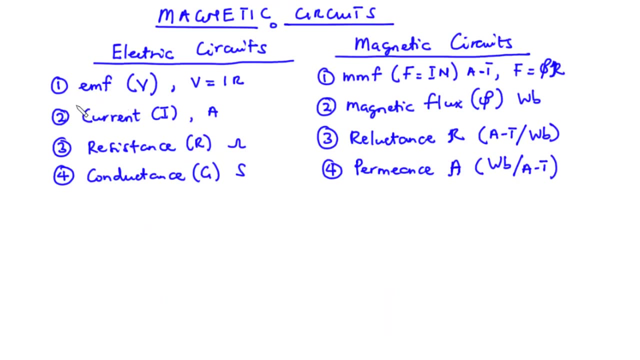 permeance is defined as the measure of the ability of a material to permit the setting up of magnetic flux. So, in summary, in an electric circuit we have the source to be the EMF, that is, the electromagnetic force, and then represented as V, and that is equal. 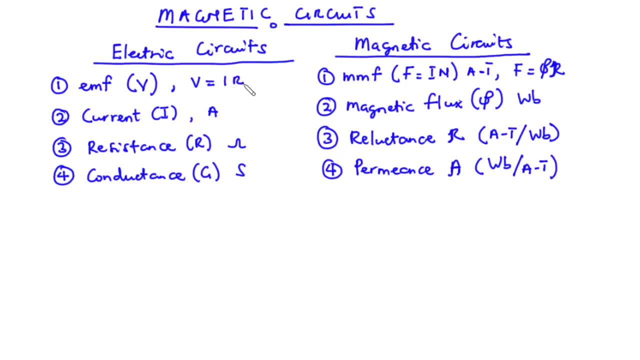 to the current flowing in the circuit times, the resistance of the circuit. Now in a magnetic circuit we call the source the magnetomotive force, and that is represented as F and given as I times N, and that is measured in amperes or ampere tens, and that is also equal to the 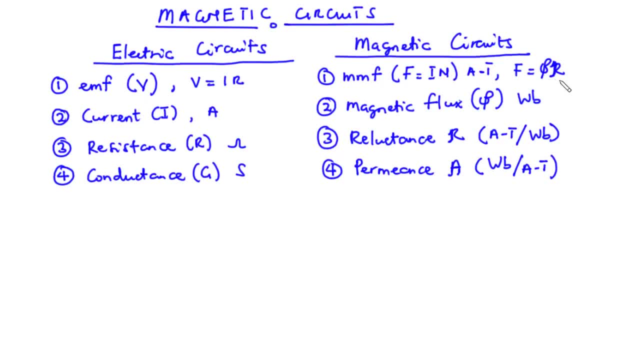 magnetic flux times the reluctance of the circuit. Now the current in an electric circuit that is represented as I, is measured in amperes and then in a magnetic circuit. we call that the magnetic flux and that is measured in webes, Also in an electric circuit. the opposition. 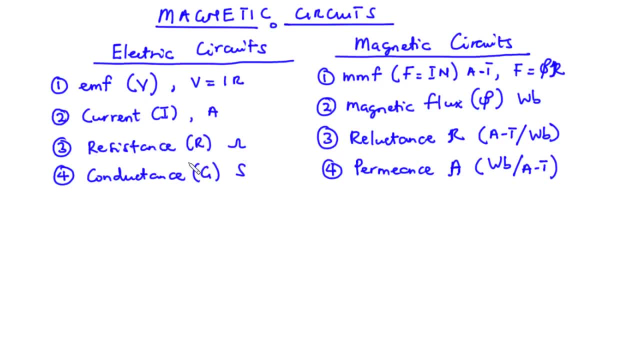 offered to the flow of current is called the resistance. that is represented as R and then measured in Ohms Inside of a magnetic circuit. we call that the reluctance, that is, the opposition offered to the flow of magnetic flux. that is also represented as R and is measured in. 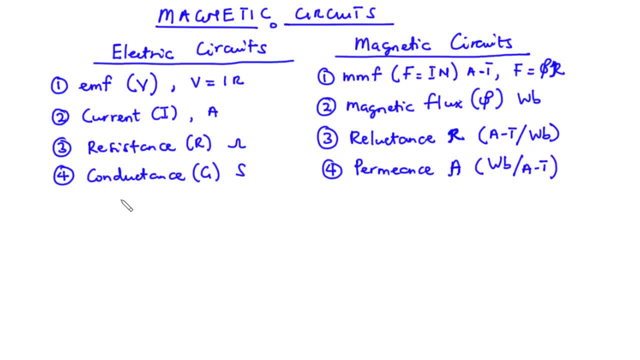 ampersands per webes. The conductance in an electric circuit, which is represented by g and then measured in Siemens, is called the permeance in a magnetic circuit. that is also represented by A and that is measured in Weber's pair ampere-tens. So that's it. 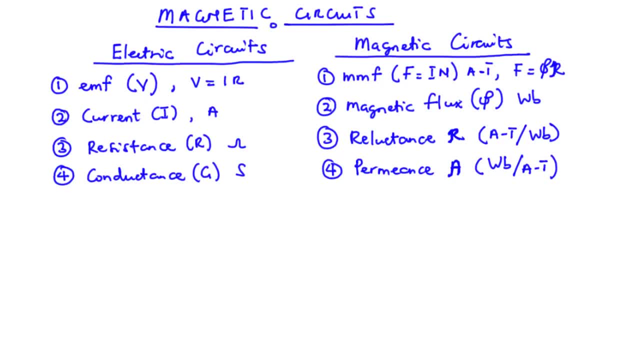 for today's video. Thanks for watching and see you in my next video. Bye, bye. 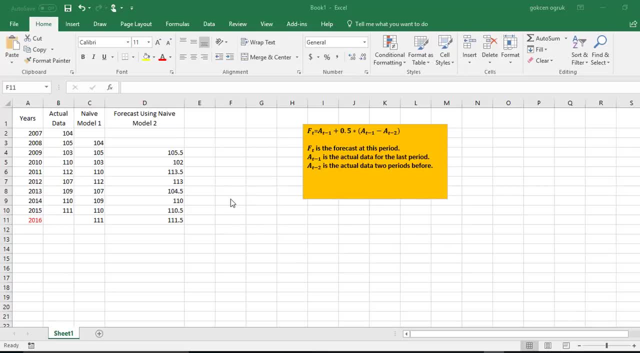 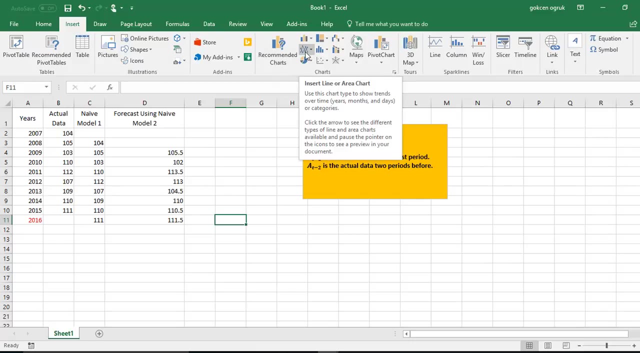 Hi everyone. In this video I'm going to show you how to plot multiple lines on an Excel chart. So to do that we need to just click on an empty cell And after that I'm going to click on insert. From insert I will come here for insert line or area chart. 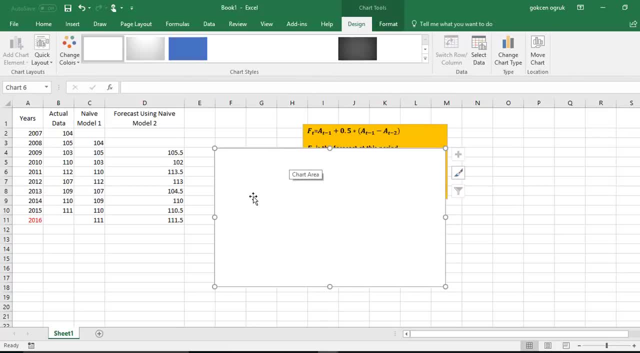 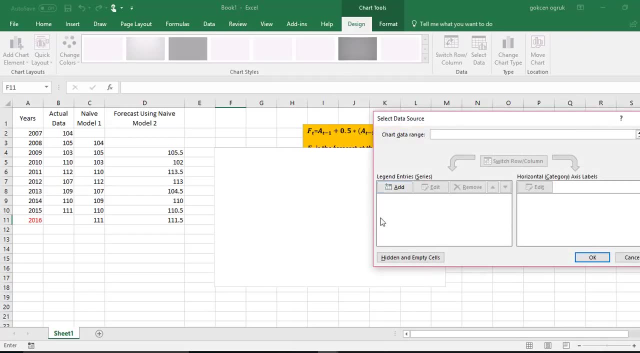 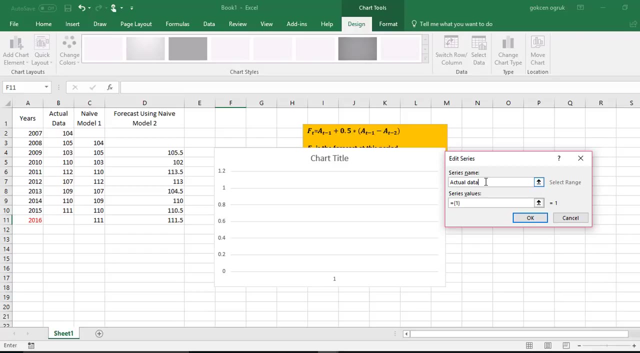 And then I will choose the first one. Now you will see an empty chart area. We need to add the data to this chart area. Right click on the mouse, select data, And then I will start with add. Now I need to title my series, which I will say actual data.